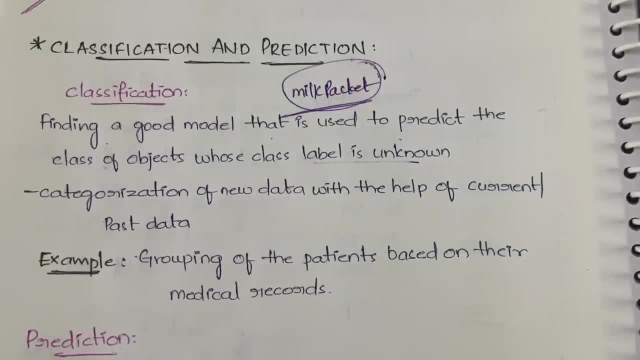 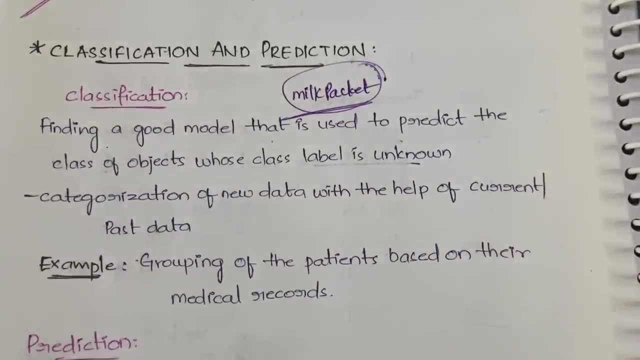 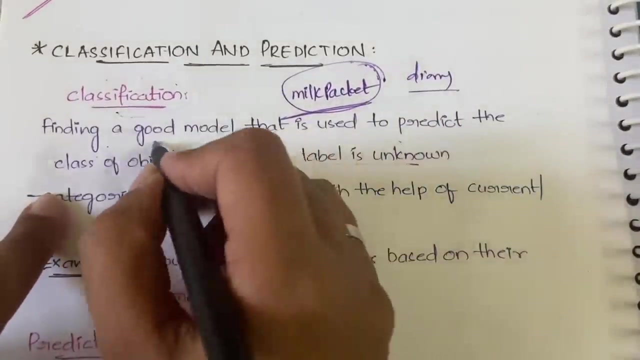 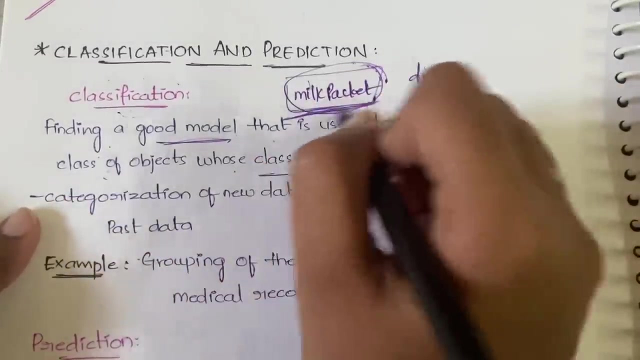 which category in the supermarket. You don't know to which category this milk packet belongs to. You don't know where. you have to keep it right. Then how do you place it in a dairy section? Actually, it is supposed to be in the dairy section, right? So this classification will help you in finding a good model that is used to predict the class of objects whose class label is unknown. If you don't know that, the class label of this, that is where to place this object. you don't know that. 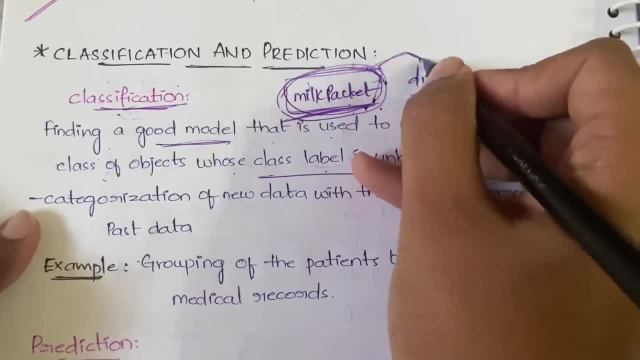 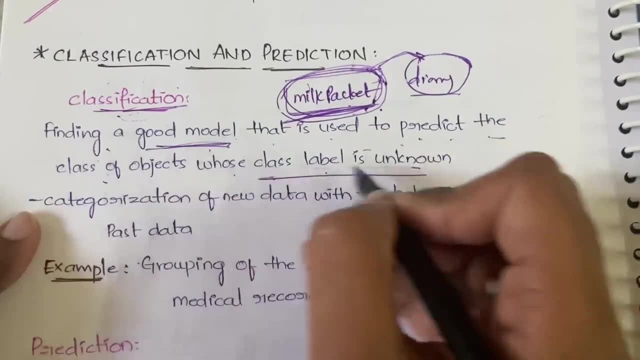 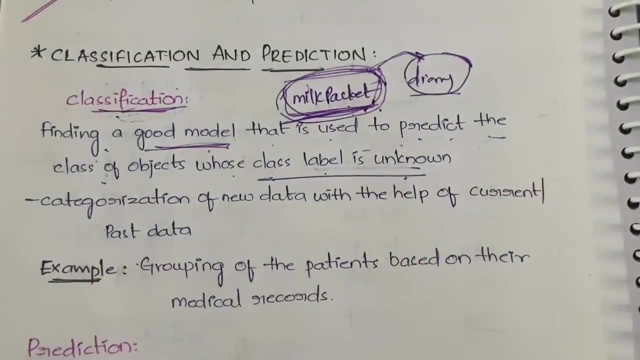 then the classification will help you out in placing this object in the appropriate position. Here also the same: finding a good model that is used to predict the class of objects whose class label is unknown. Now, what is the model that you are using to place a milk packet in the dairy section that milk belongs to, or milk is a dairy product. it will be written on the packet that it is a dairy product or something like that, right So in the example. I'll tell you one more example where you'll understand more clearly. classification is nothing but simply. 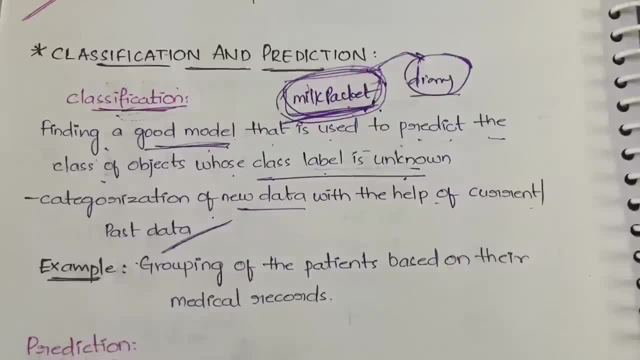 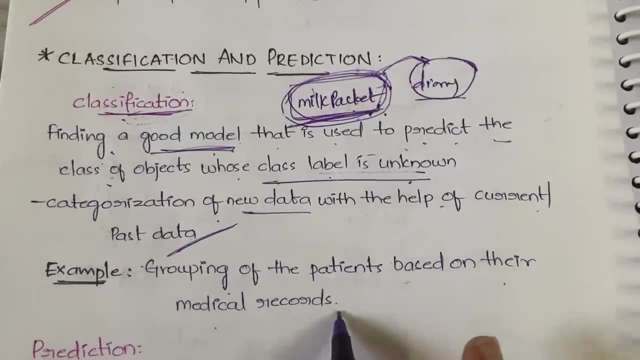 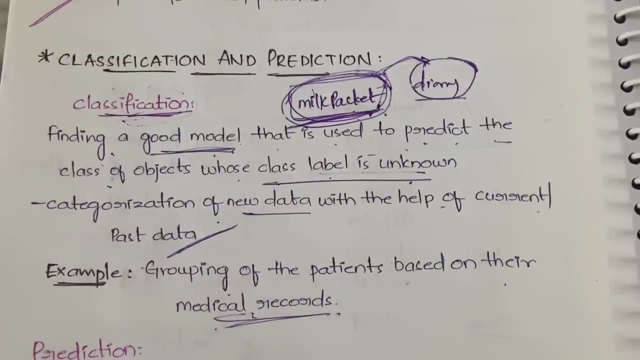 of the new data with the help of the current or the past data is called as the classification. That's all. you're dividing the newly coming data into different, different categories based on the previous data or the current data. that is called as classification. Example: grouping of patients based on their medical records. that is based on the medical records. you are grouping the patients like what is the previous history like- if they are having any BP, sugar, diabetes or sugar or diabetes, anything the same- And 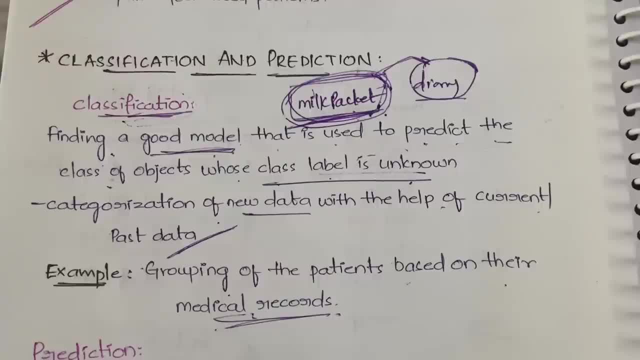 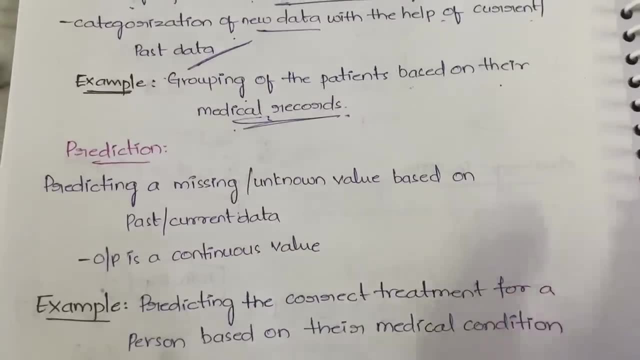 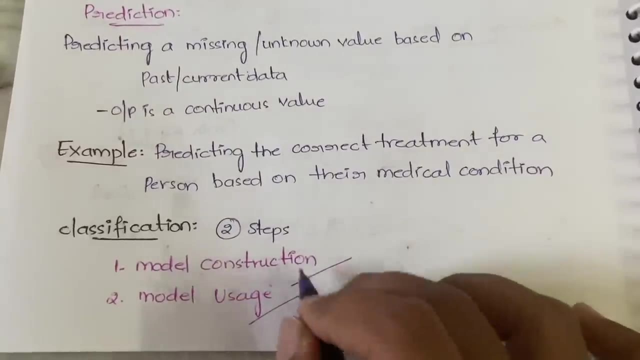 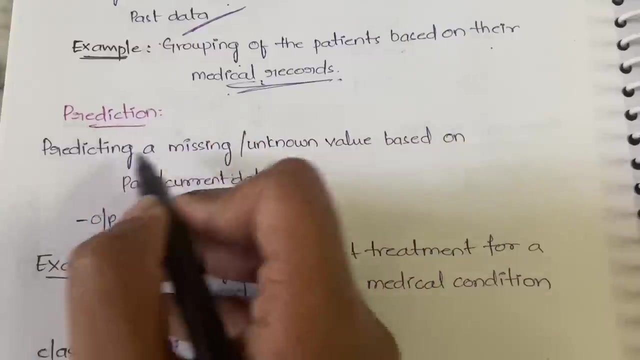 the cholesterol or thyroid. So, based on the medical records, you are grouping the patients. Okay, that is the classification. Don't worry about classification. I'll tell you one more example- pass or fail example. that will be more clear for you. We actually have two steps in classification: model construction and model usage. Okay, I'll tell you what is model construction and model usage was before that. let us complete prediction. Prediction is nothing but the word itself says predicting, predicting a missing or unknown value based on the medical records. you are grouping the patients. Okay, that is the classification. Don't worry about classification. I'll tell you one more example- pass or fail example. that will be more clear for you. We actually have two steps in classification: model construction and model usage. Okay, I'll tell you what is model construction and model usage was before that. let us complete prediction. Prediction is nothing but the word itself says predicting, predicting a missing or unknown value based on the medical records. you are grouping the patients. Okay, that is the classification, Don't worry. 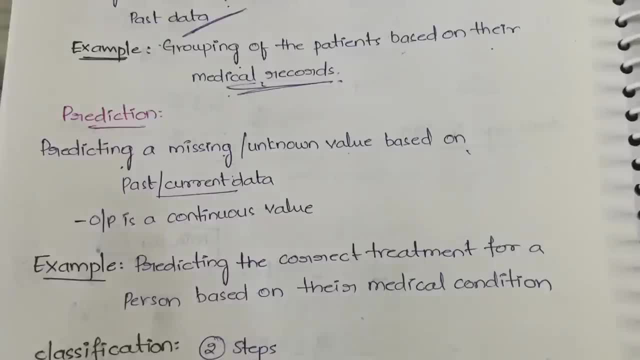 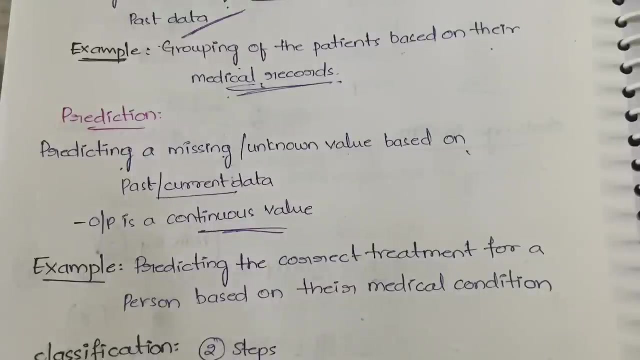 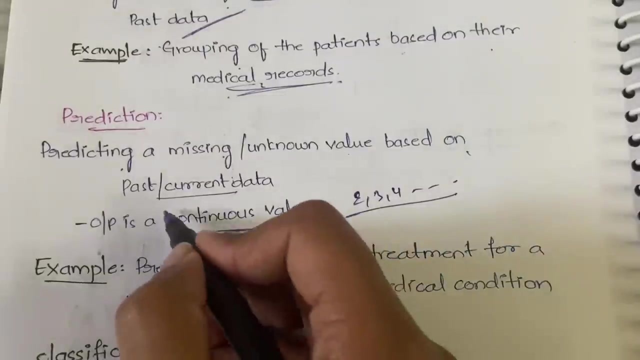 on the past or current data is called as prediction. you any missing value or unknown value. you are predicting it. How are you predicting it? based on the past data or the current data? you are doing the prediction, got it, and the output which you get is a continuous value, not a discrete value. discrete value in the sense individual, like 234, it is not an individual value. Okay, they are not discrete values. The output which you obtain is a continuous value. continuous intervals: data will be in continuous intervals. 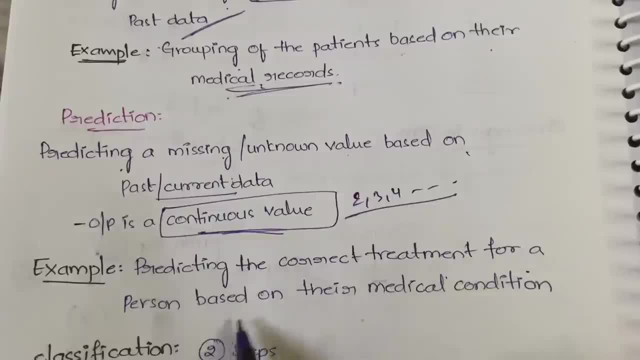 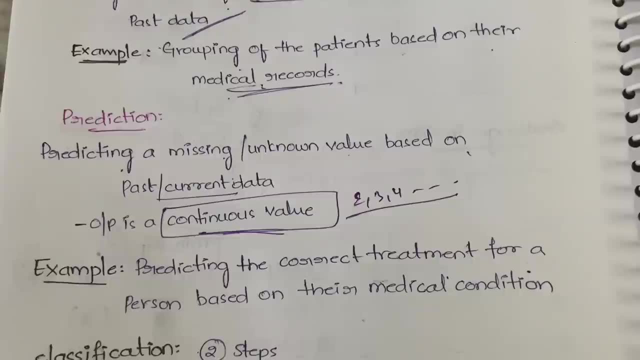 Okay, got it. example: predicting the current rate correct treatment for a person based on their medical condition. So, based on the medical condition of the person, that the person is, you know. if the diabetic levels of the person is high, then you will identify that. okay, this person is a diabetic, So we have to give him relevant medicines. Okay, like that you will be identifying, you will be predicting what treatment has to be given to the patient based on the medical condition of the patient, got it? that is prediction. 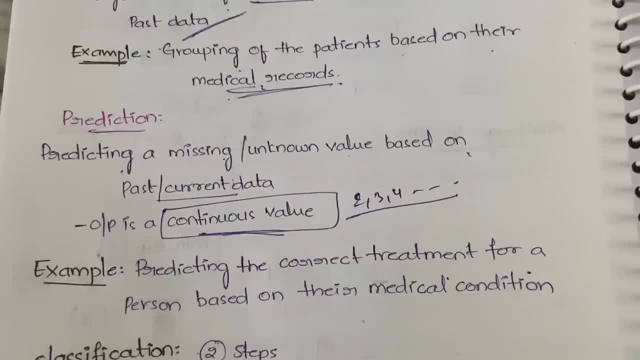 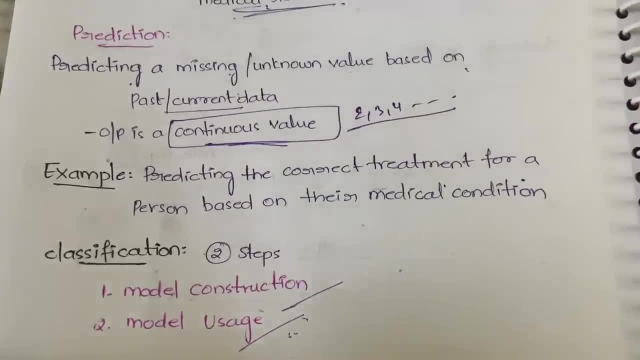 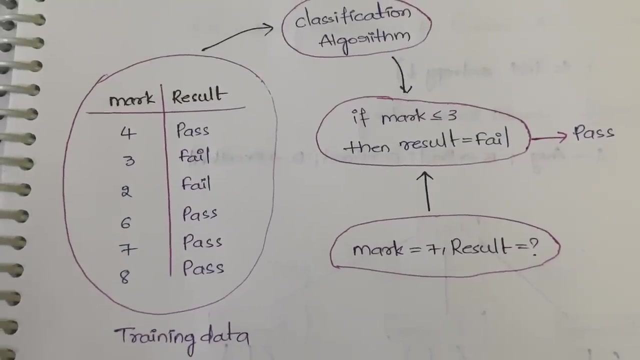 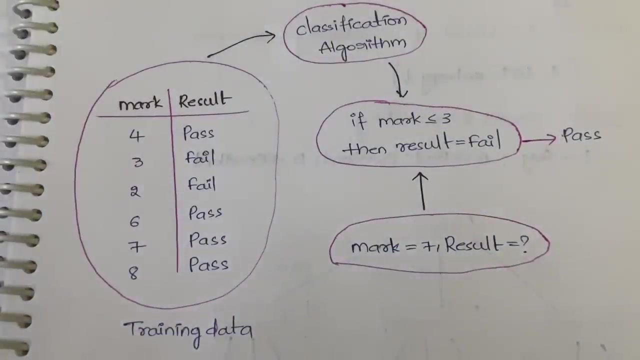 Okay, so this is about classification and prediction. Now, as I said, in classification we have two steps, So I'll tell you what are those two two steps: model construction and model usage. Both of them I'll show you in a single diagram. So this is the diagram. Let me zoom in a bit. Yeah, this is fine. So, mainly here, what you have to remember is this is the training data marks and 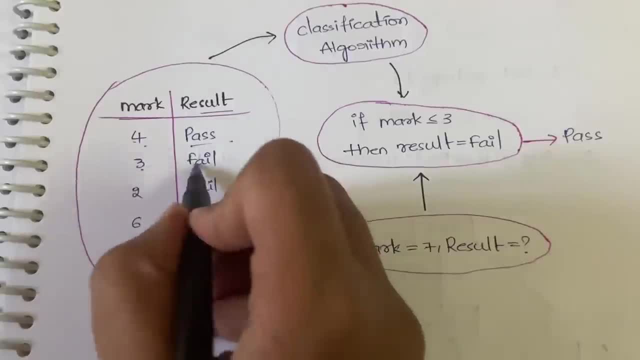 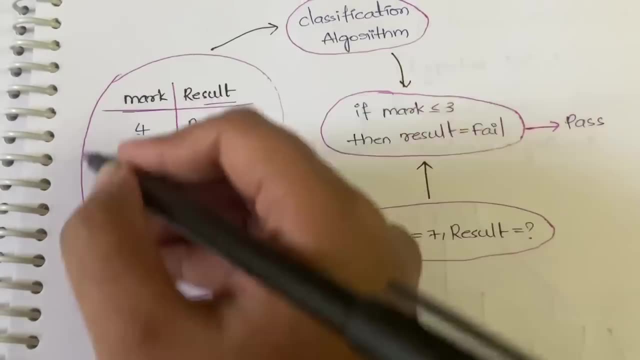 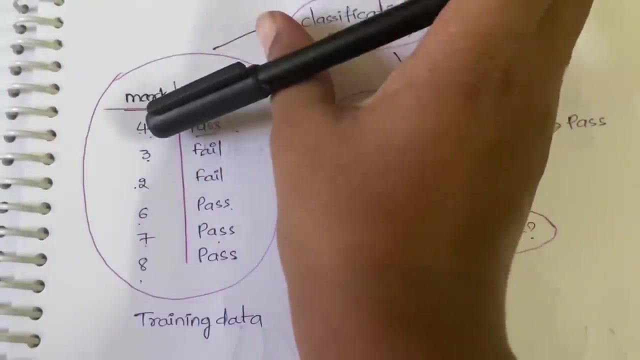 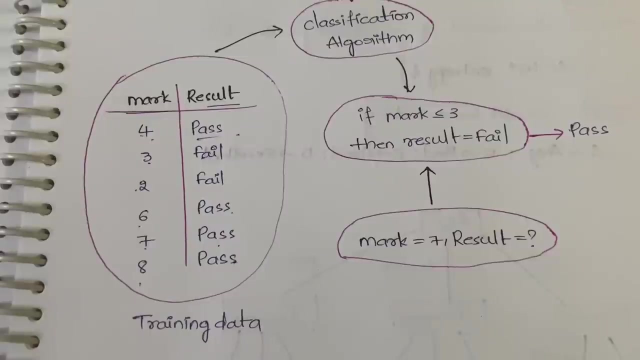 result are given. If the mark is four, then the result is pass. If it is three, it is fail. If it is two, it is fail. If it is six, it is pass. seven pass, eight pass. So this is the training data which will be given to the classification algorithm. Okay, the training data will be sent to the classification algorithm. Why? Because the algorithm has to learn. See if you, if suppose you're writing max exam, max. So in max exam you are having some calculations. 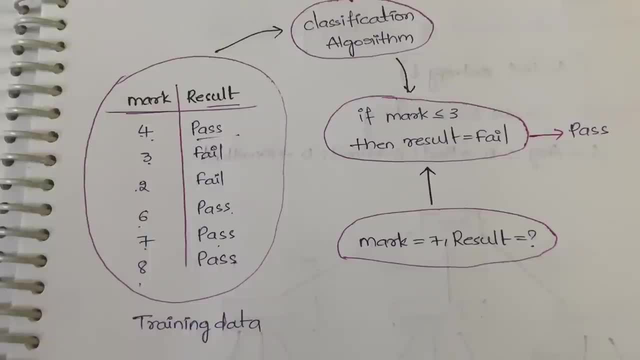 Simple calculations only, Then in that case you have to prepare some problems and go right. So if you prepare some problems and go, even though if there are some numerical changes, or even though if there are some changes in the names of the persons in the problems, like in word problems or numerical changes, then you can do the problems because you have already learned them. you know the model, you know the process, how to solve it Right. So here also, first the algorithm. the classification algorithm will learn from the 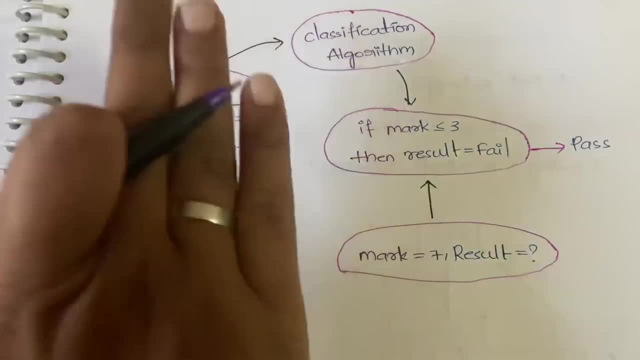 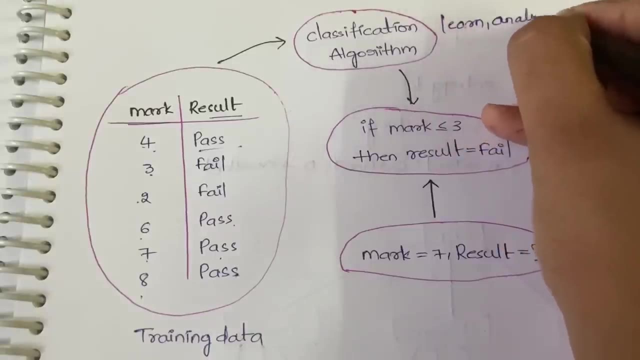 training data. Okay, this is the original data, initial data. we have the classification. will learn. it will learn, it will analyze and it will generate. Okay, and it will generate the classifier model. Okay, it will generate the classifier model. classifier model is nothing but this one, Okay. 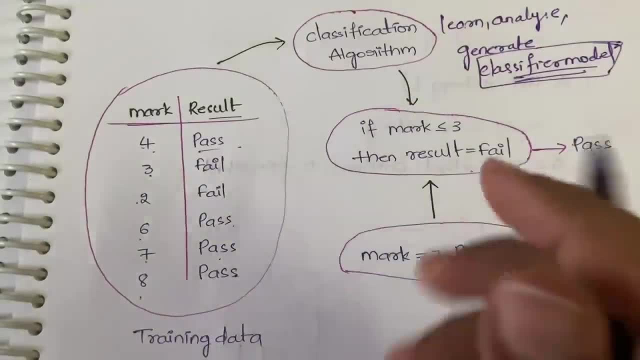 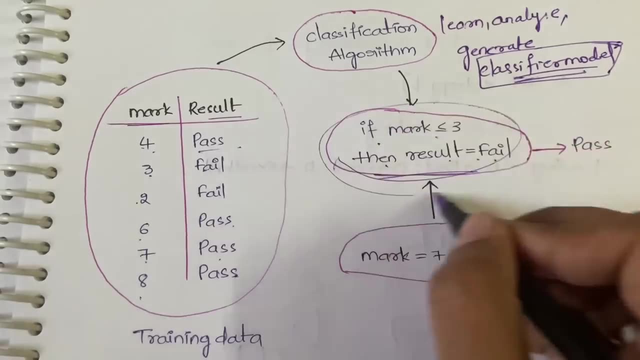 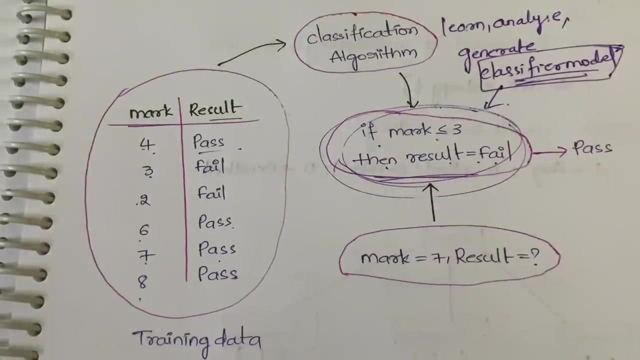 the main classification of data is being done on. done because of this one only right. if the mark is less than or equal to three, then result is equal to fail. So the main classification is happening only because of this thing. So this is the classifier. model Got it. This will be doing the classification. So till here, it is said to be model construction. Got it? Now, whatever data is given to this model, whatever input we are giving, this is our input. 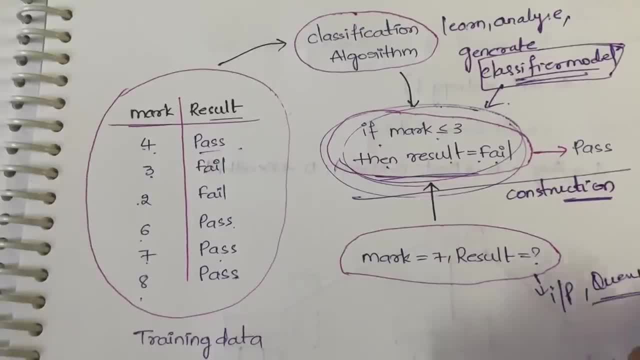 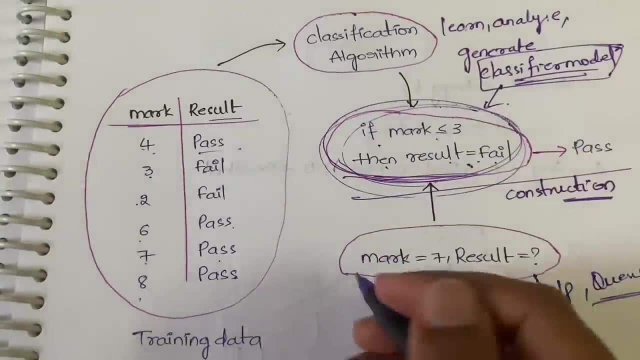 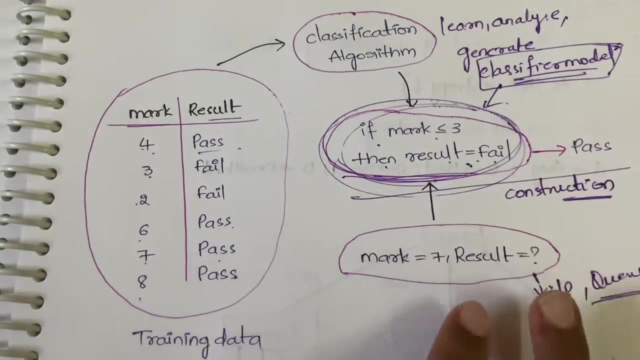 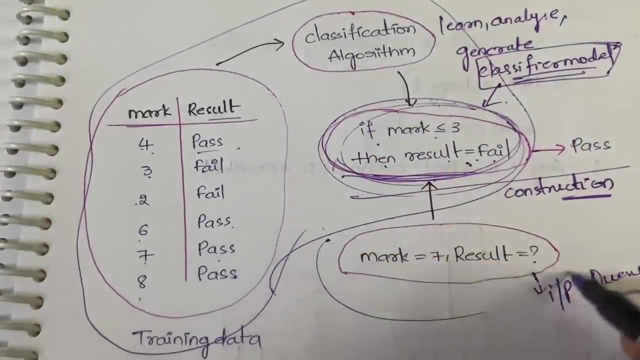 Okay, whatever input or query you can say is being given to this model, based on the condition it has, it will give the data, it will classify the data. This is called as model usage. You are, you have created a model, And now you are using that model. that is called as a model usage. Till here, what you did? this all is about creating a model, So it is called as model construction. Here what you are doing: you are using that model which you have constructed, Got it. So here, 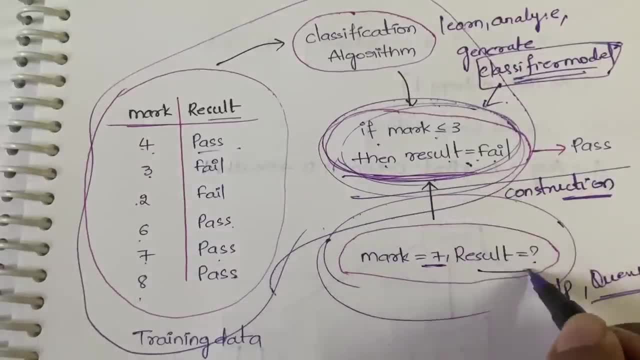 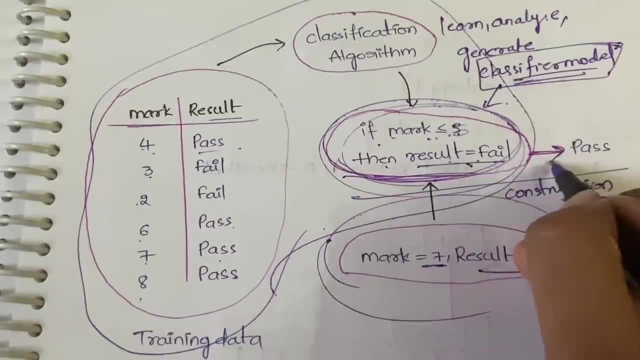 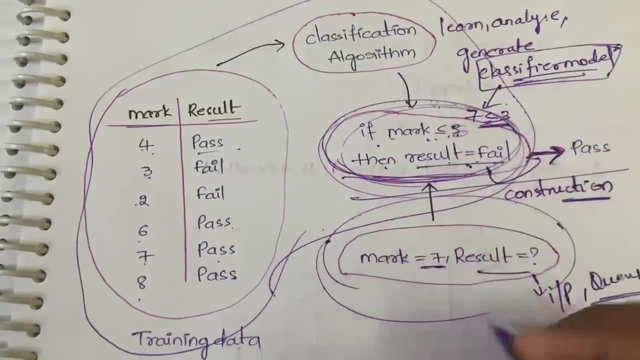 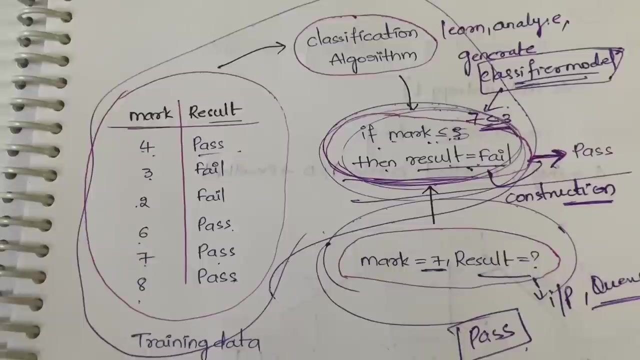 you are giving Mark is equal to 7. Then result is equal to how much? So, according to the condition, If the mark is less than or equal to three, then the result is equal to fail. else it is pass. So Mark is seven is less than or equal to three, Is it true? no right, so it will directly come out and the result will be printed as pass. Got it? This is how this will work, Got it? This is all about this video: classification and prediction in classification. 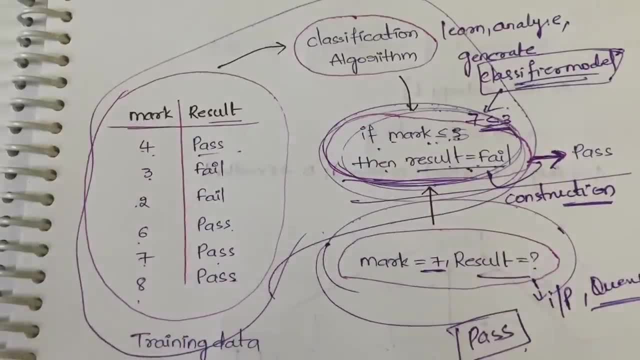 we have two steps: model construction and model usage. So this is all about this video. thanks for watching the video till the end. and we have different classification algorithms as well. we will be seeing in the next coming videos like we have decision tree, we have patient classification, we have rule based classifier and so on. okay, we will. 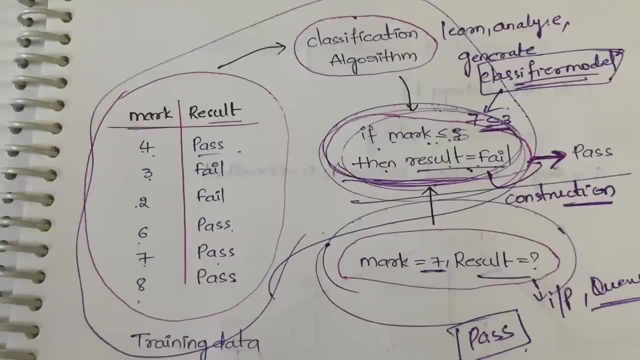 be learning them in the next coming videos. thanks for watching the video till the end. if you're still having a doubt, just let me know in the comment section. i'll definitely try to clear all your doubts. for sure. make sure that you subscribe to this channel so that you can get any notifications. 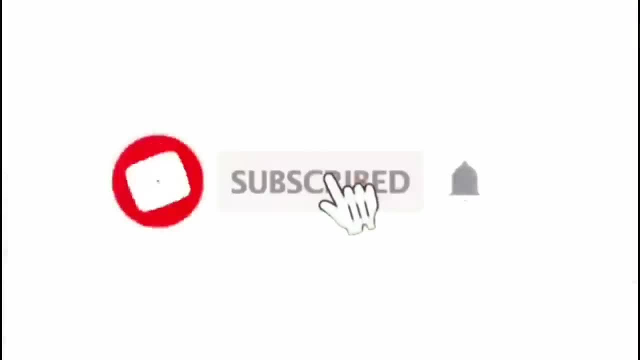 whenever i post a new video. thanks for watching the video till the end you. 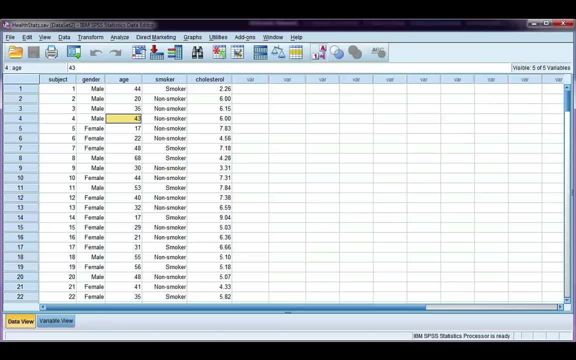 We're going to look at how to run a chi-squared test in SPSS and interpret the output. Now I've got a database with some health statistics and we're going to use gender and smoker or smoking status, so whether the person's a smoker or a non-smoker. Now the reason I'm 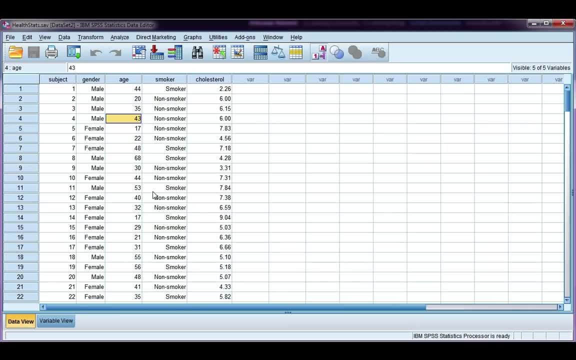 going to use these two is because we usually use a chi-squared test when we have two nominal variables. Now, remember, nominal is data that has no meaningful rank or order. so smoker, non-smoker, male, female, They're definitely nominal variables. So let's go to analyze. 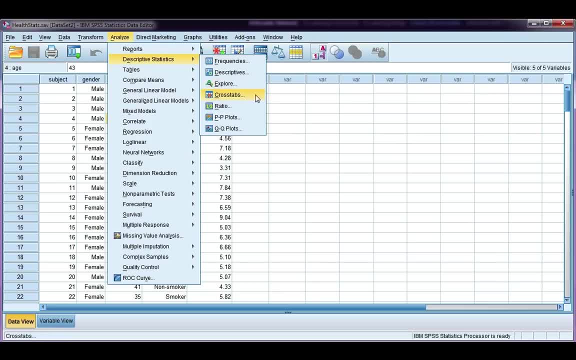 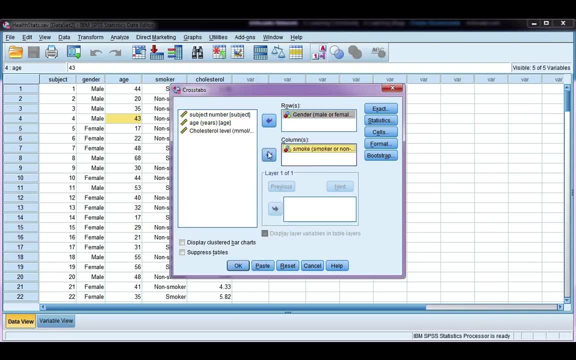 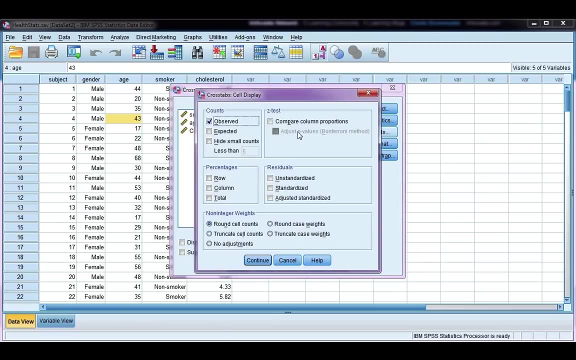 descriptive statistics and crosstabs. I'm going to reset and I'm going to put in gender and smoker. It doesn't really matter which way around you do it, I've just chosen to put it this way. We're going to go to cells and I want to show you the expected count.